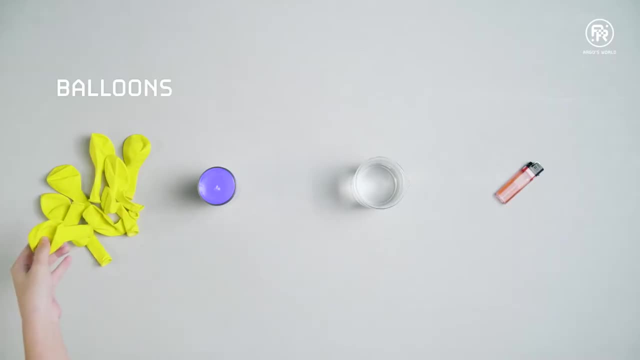 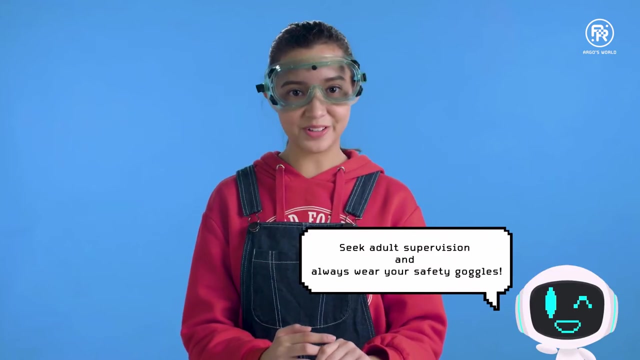 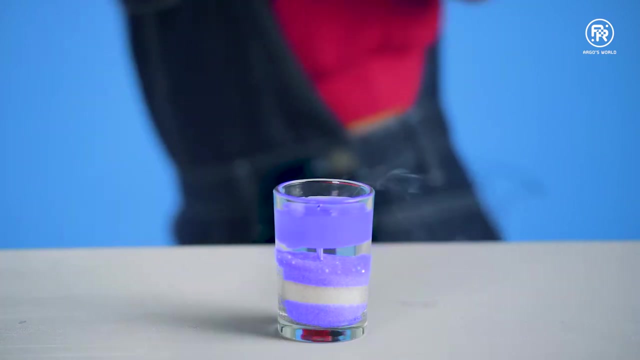 this experiment you'll need some balloons, a candle, some water, a lighter or matches. First, light up the candle and blow up your balloon. Tie the balloon securely. What do you think will happen when I place the balloon over the flame? Yes, it pops. This happens. 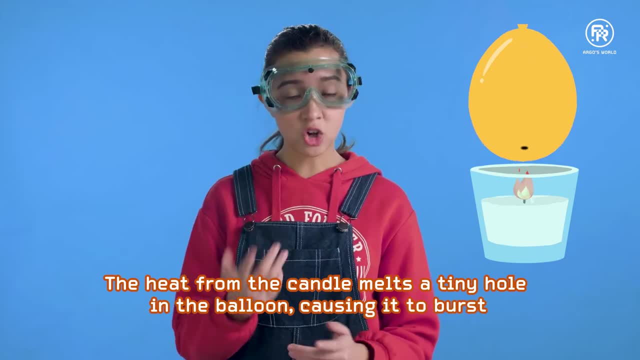 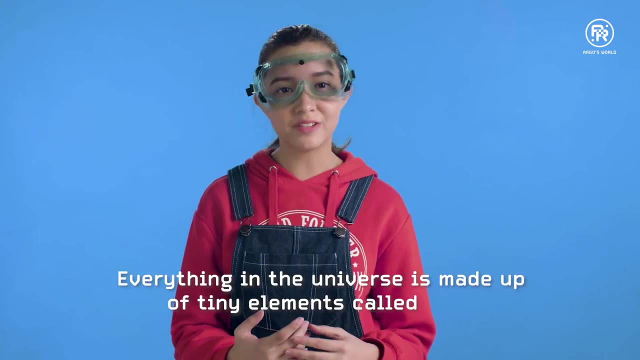 because the heat from the candle melts it through the flame. When the balloon is hot, a tiny hole in the balloon causes it to burst. To understand why this happens, first you need to know that everything in the universe is made out of tiny elements called atoms. When something gets hotter, its atoms move faster and away. 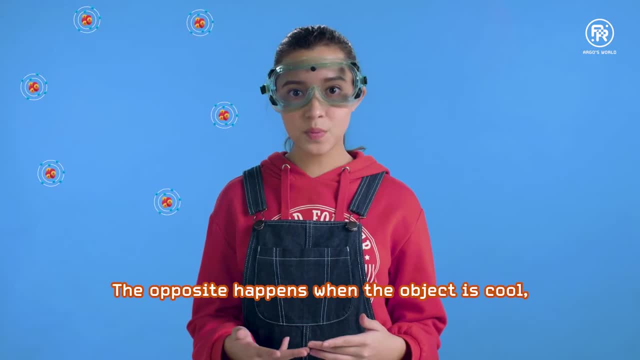 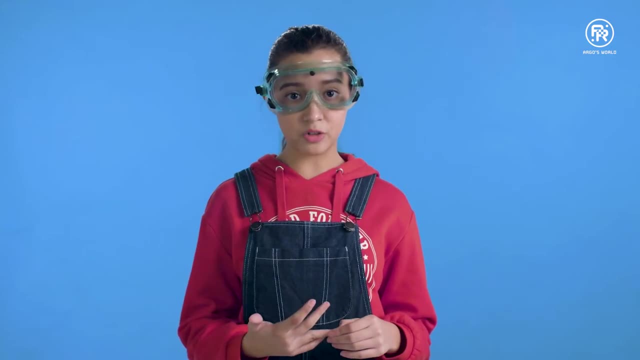 from each other, making the object expand. The opposite happens. when the object is cooled, The molecules slow down and the object contracts. We can usually prevent the balloon from popping by putting some water inside. Let's try it again now. We'll hold the balloon. 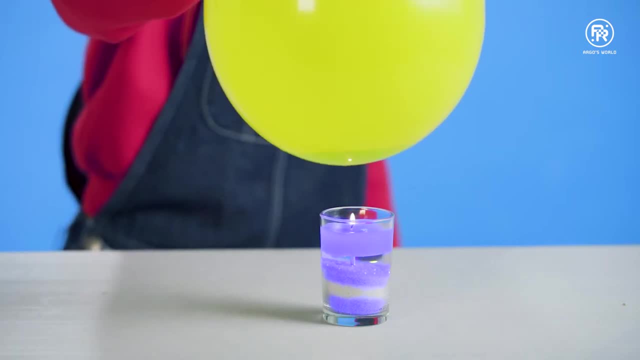 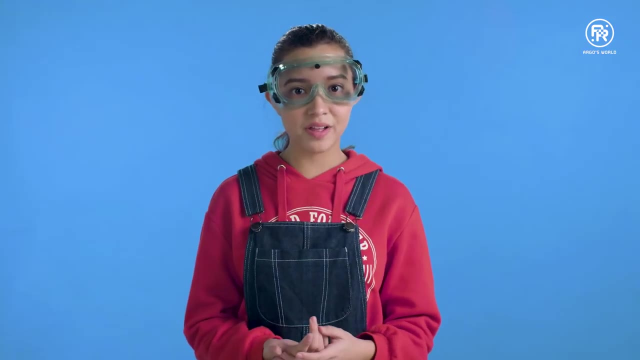 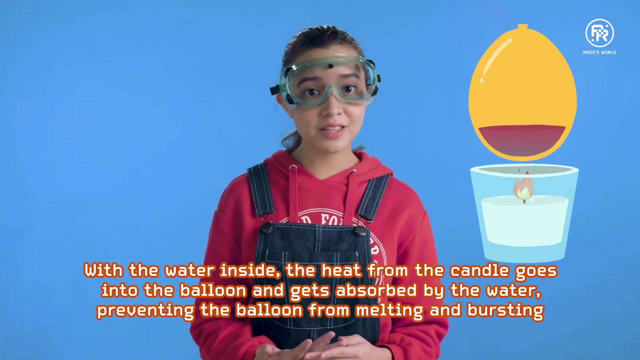 with water over the flame for about five seconds- One, two, three, four, five- It didn't pop. With the water inside, the heat from the candle goes into the balloon and then it is absorbed by the water, preventing the balloon from melting and bursting. Now I'm going to place 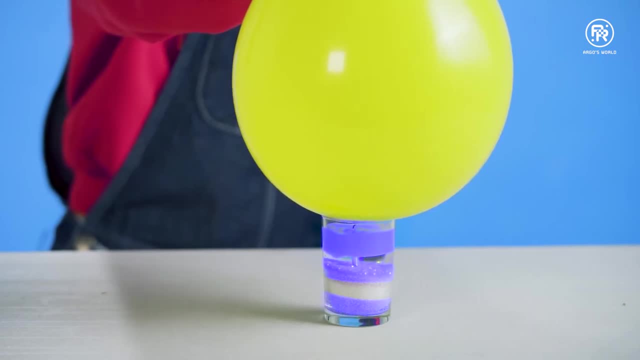 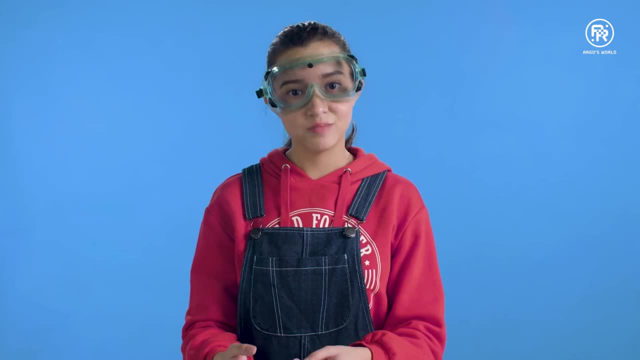 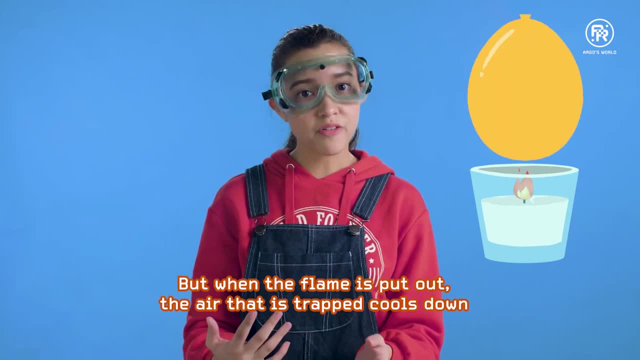 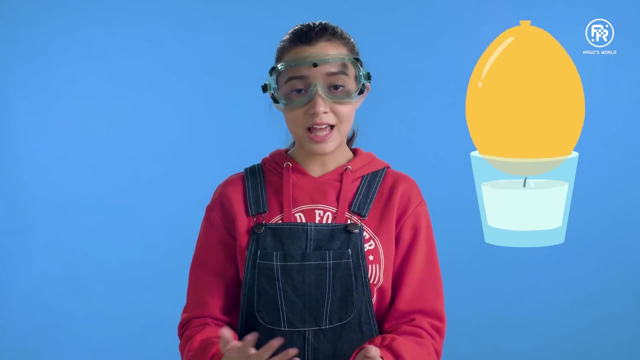 the heat energy expands the air molecules around it, But when the flame is put out, the air that is trapped cools down, The molecules contract and the suction pressure is created, allowing me to do this. Energy exists in many different forms. There is heat energy, which 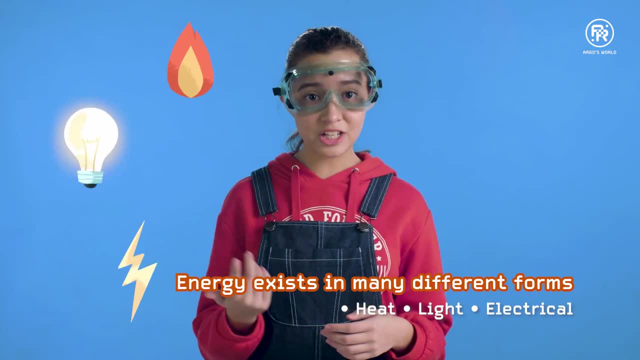 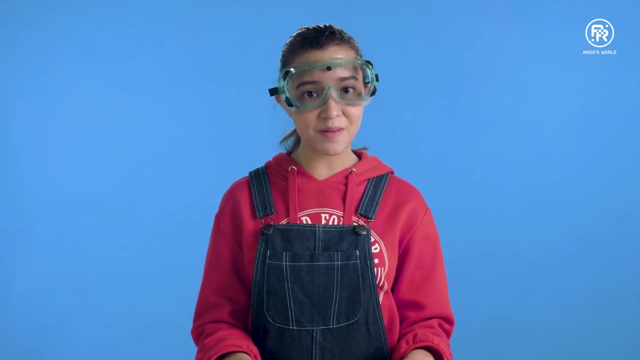 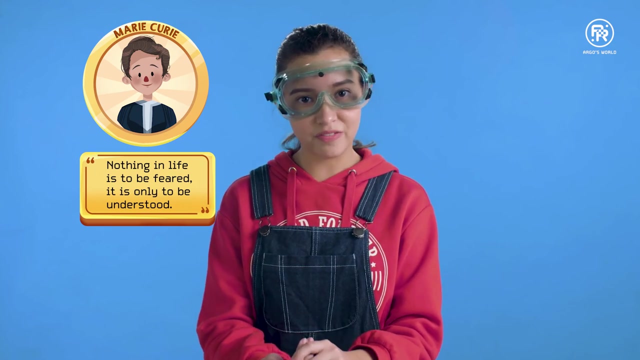 we just explored today: light energy, electrical energy, sound energy, kinetic energy and lots more. What other fun experiments can you do to demonstrate transfer of energy? As my favorite scientist, Marie Curie, once said, nothing in life is to be feared, It is only to be understood.